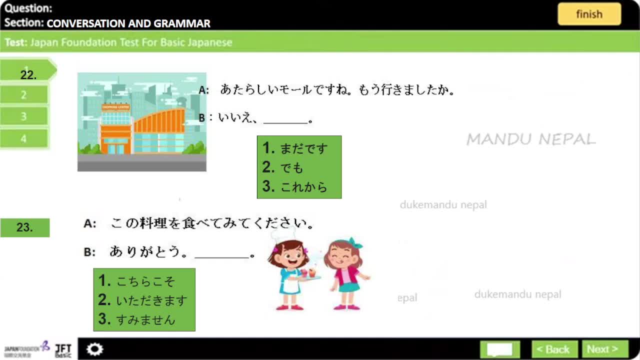 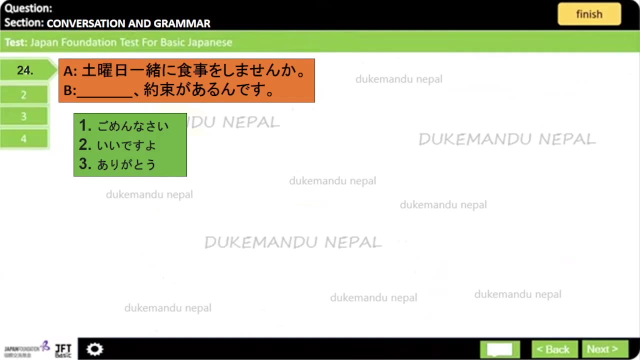 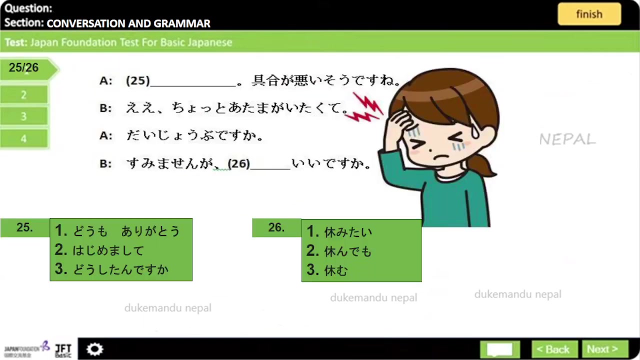 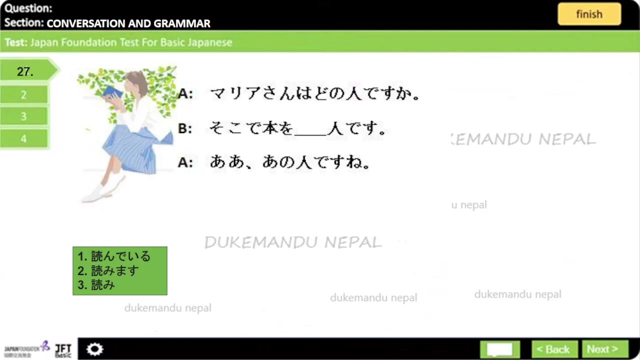 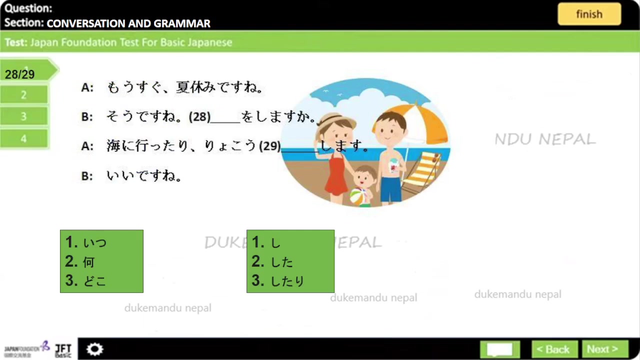 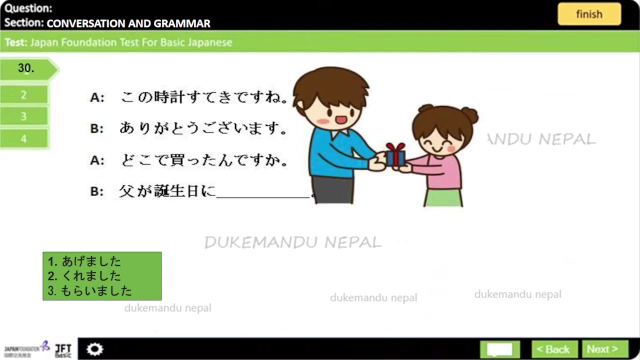 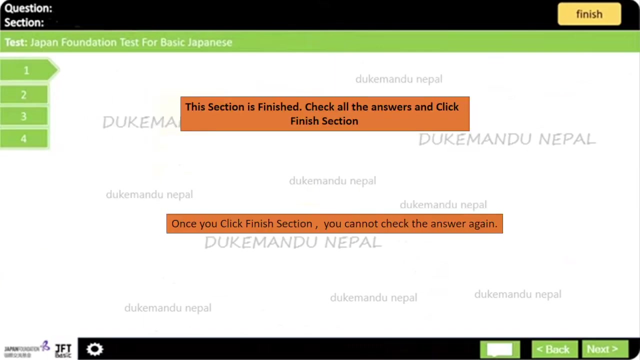 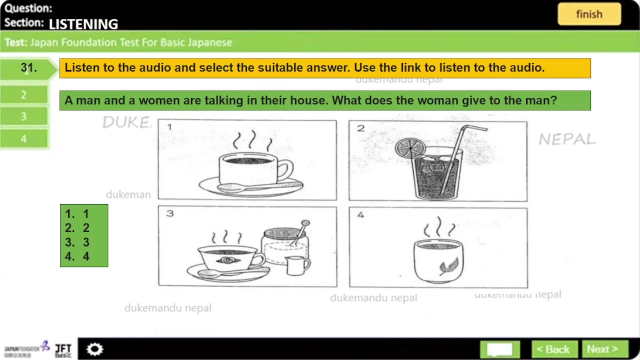 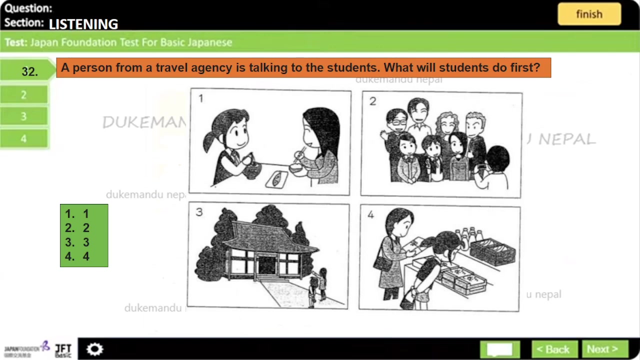 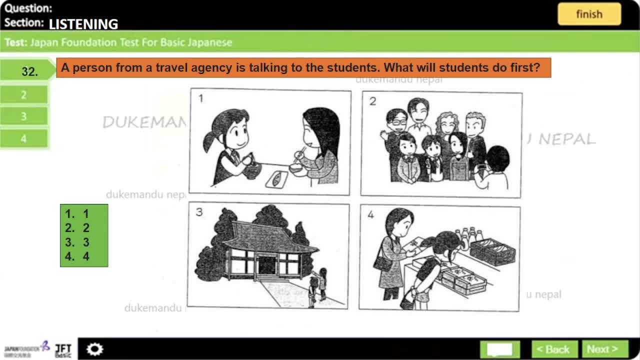 ご飯を食べたり、お寺を見たり、買い物をしたり、好きなことをしてください。 2時にまたここへ来てください。 では、写真を撮りましょう。. 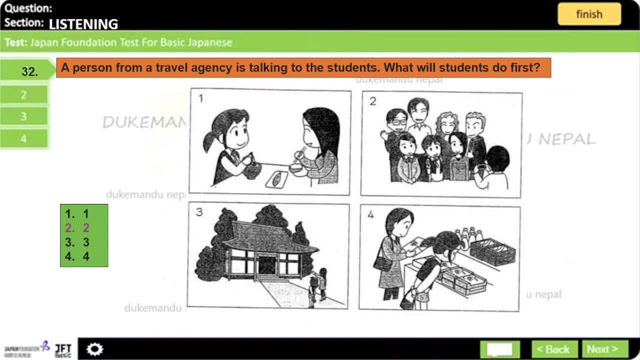 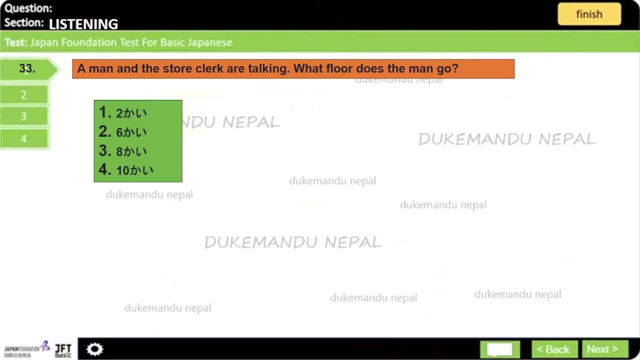 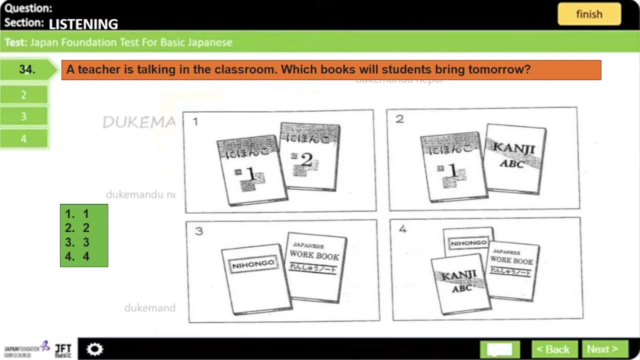 2時にまたここへ来てください。 明日から日本語のクラスが始まります。 この日本語1は毎日使いますから、 忘れないでください。. 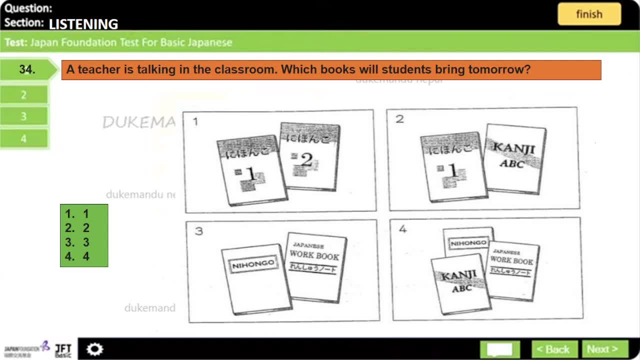 2は今は使いません。. それから、明日は火曜日ですから、漢字の授業もあります。 漢字の本も持ってきてください。 先生、この本は. 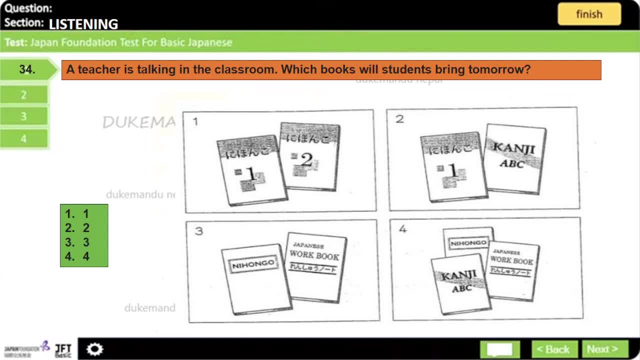 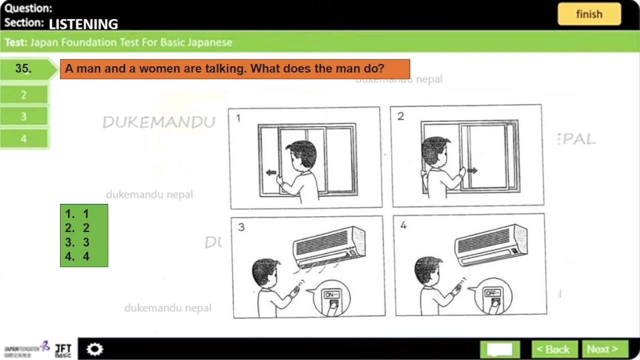 その本は練習に使う本です。 家で使ってください。 この部屋、暑いですね。 そうですね。 窓を開けましょうか。. 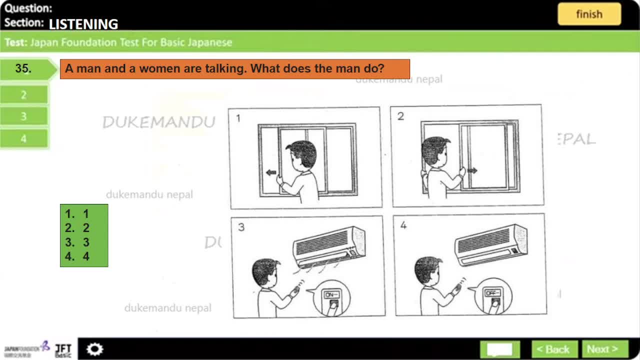 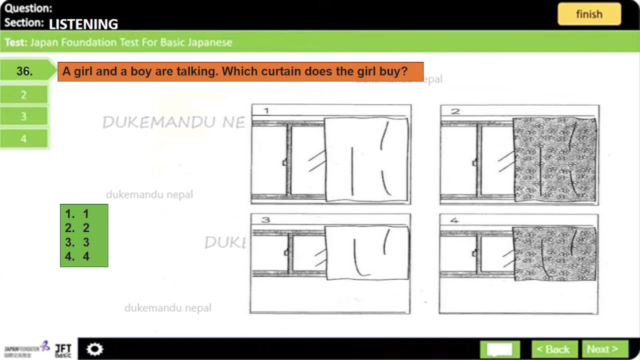 いいえ。 今日は風が強いですから、窓は開けないでください。 エアコンをつけましょう。. そうですね。 明日は何をしますか? 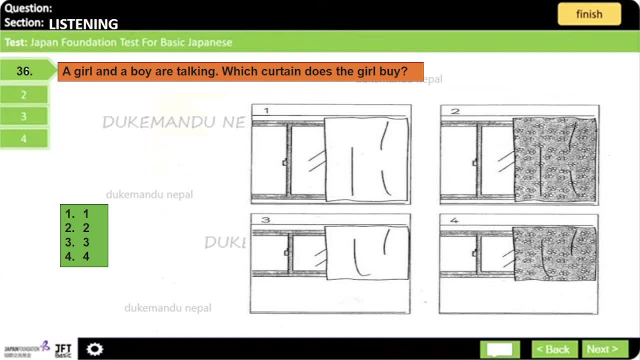 カーテンを買います。 カーテンを 小さいカーテンですか? いいえ、大きいカーテンです。 私の部屋に最初からありましたが、あまり好きなデザインではありませんでした。. 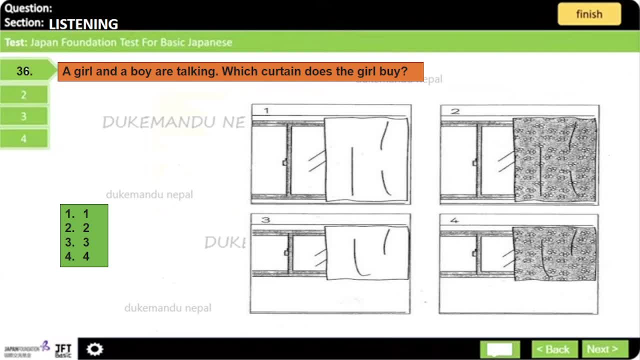 花の絵で。 そうでしたか。 どんなカーテンにしますか? 白で何も書いていないものにします。 カーテンを買います。. 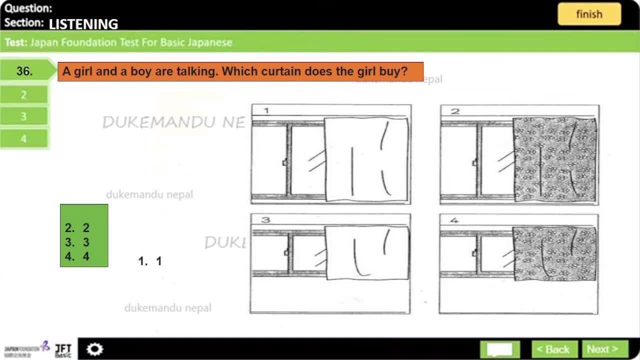 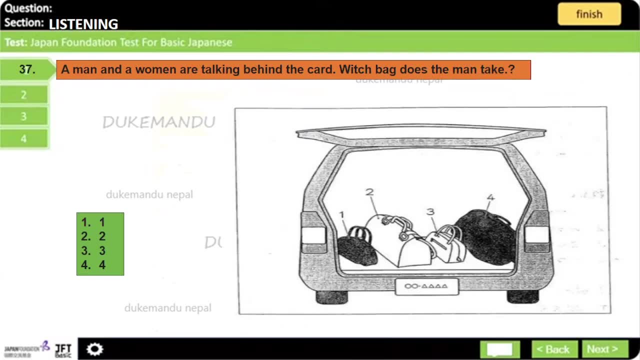 カーテンを買います。 カーテンを買います。 カーテンを買います。 あ、カーテンを買いました。 で、カーテンを買いました。. 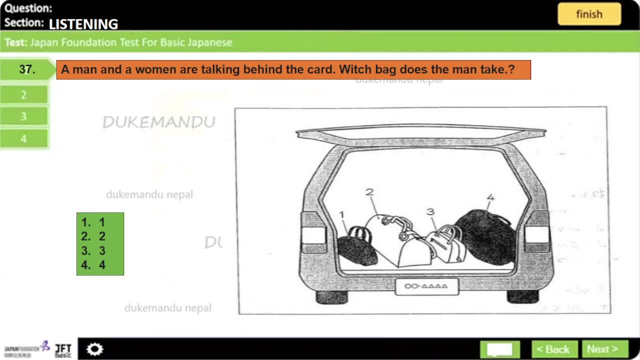 花のカーテンはどれですか? その白いカーテンです。 これですか? とそれはこれです。 ああ、これです。 結構大きいですね。. 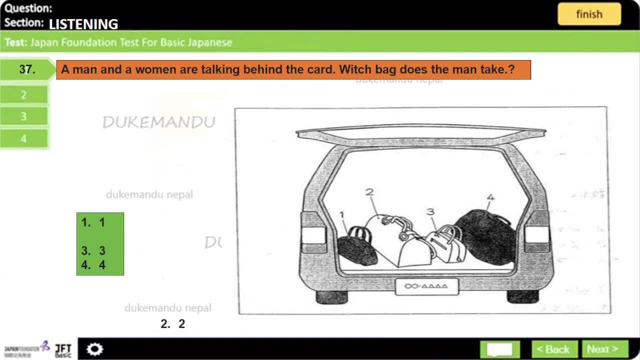 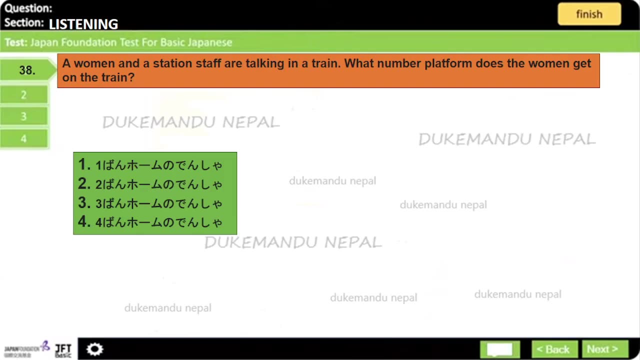 Thank you for watching. The train to Kyoto is No 3 and No 4.. No 3 and No 4, right, Yes, but today is Sunday, so the train to Kyoto will not stop at No 4.. 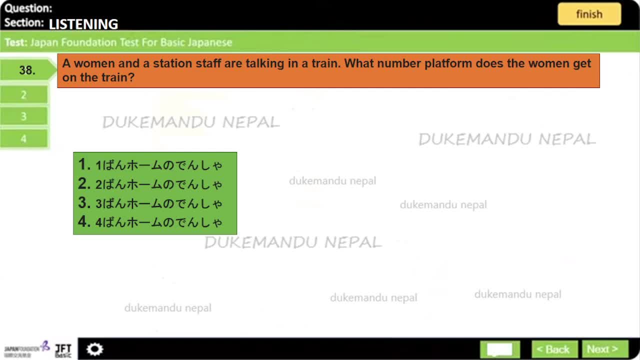 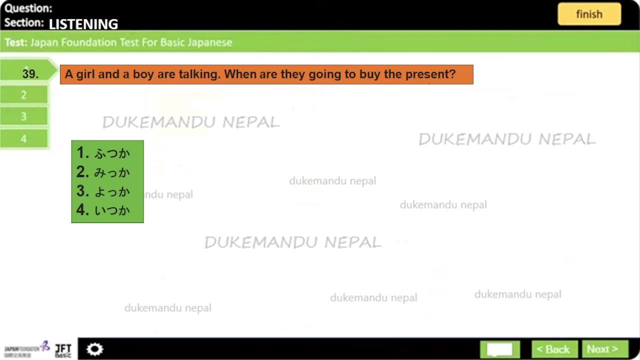 I see I understand Next week would you like to go buy a birthday present for Sakura-san? Yes, I would. It's her birthday on the 5th, so let's go on the 3rd or 4th. 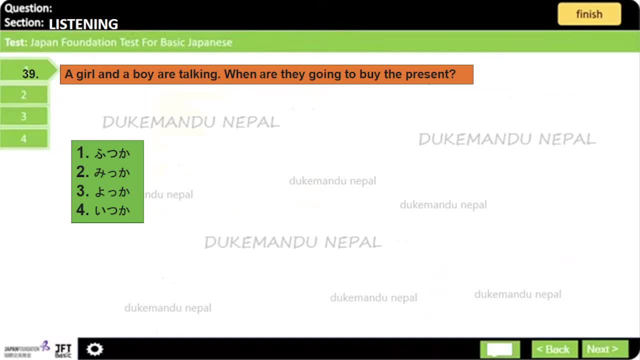 Oh, wait a minute. I have a part-time job on the 3rd and 4th. Can I go on the 2nd? Sure? Then let's go after the class is over. Two 80-yen bills please. 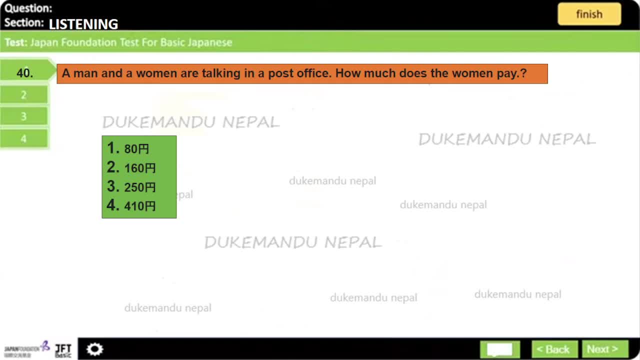 Two 80-yen bills, right, That's 160 yen. Oh, and a postcard, please. How many? Five, please. Well, five postcards are 250 yen, so that's 410 yen in total. Well, that's just right. 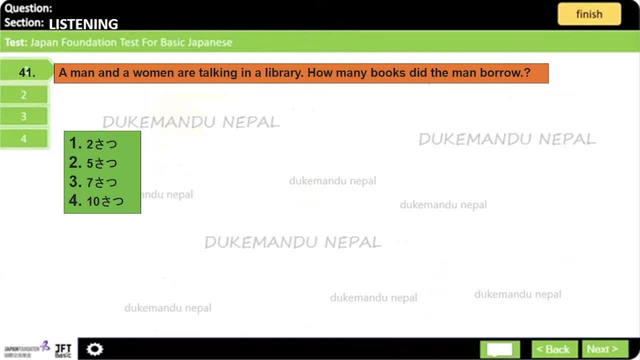 Let's see. Um, Is it okay if we pay for them? Yes, Please. There are seven postcards, right? Oh, sorry, If you're a student, you have to pay up to five postcards. What Is that the case? 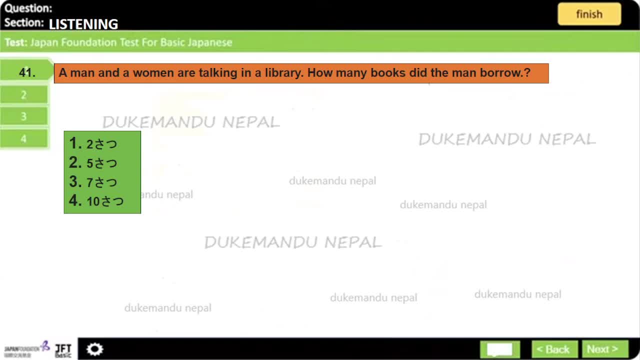 Yeah, the teacher said up to 10 books, but I understand. Then these two books are fine. Tomorrow's test is early, isn't it? Yes, it is. It's a little early at 9 o'clock. What time will Mr Tanaka come? 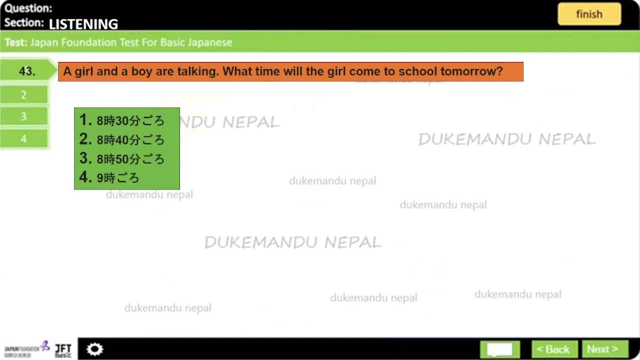 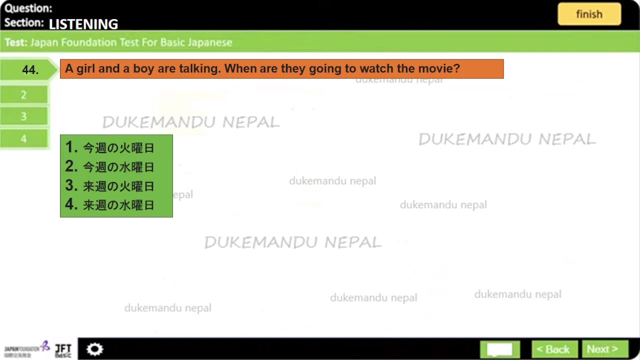 Yes, he will come about 10 minutes before the test. I see I will come about 30 minutes before and study a little. I see I will come about 30 minutes before the test. But next week will be fine. How about Tuesday or Wednesday? 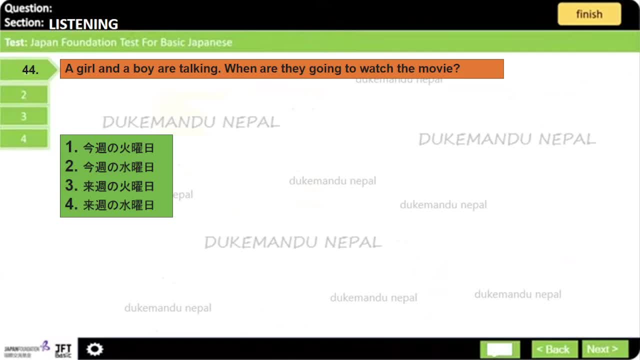 I see, Then, Tuesday is fine, Wednesday is because I have a part-time job. That's fine. Good night, Mr Yamada. what about Tuesday, Yamada? what about Tuesday? Yes, I do jogging at the park and go shopping at the department store. 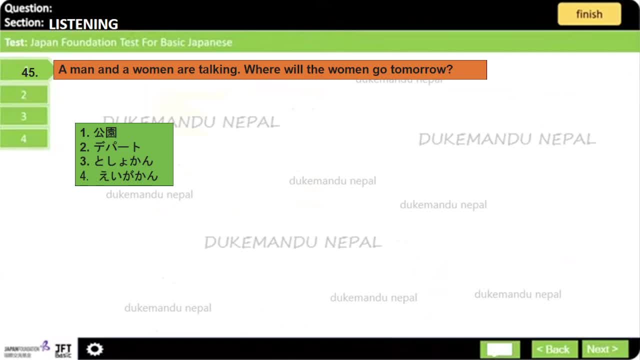 Do I What about tomorrow, Tomorrow, see you tomorrow. Tomorrow will be raining, so I may be reading books. Yes, Yes, Yes, 田中さんは, 私は友達と映画を見に行きます。. 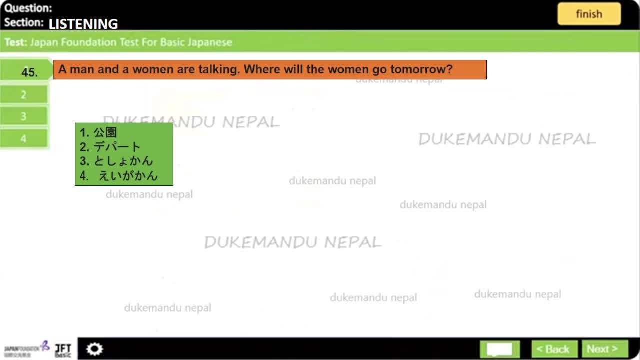 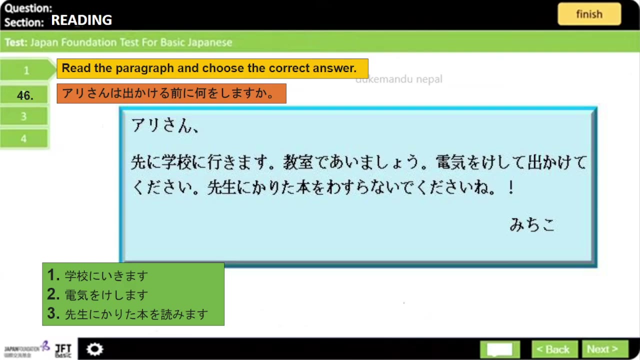 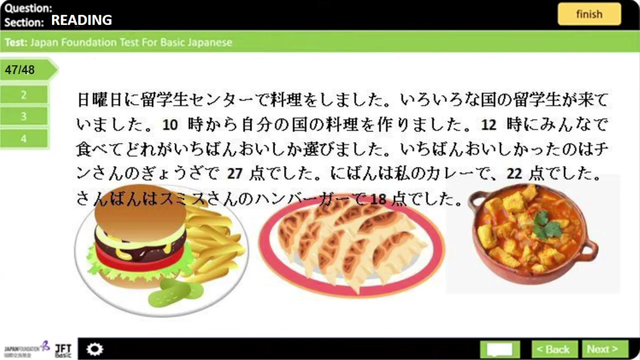 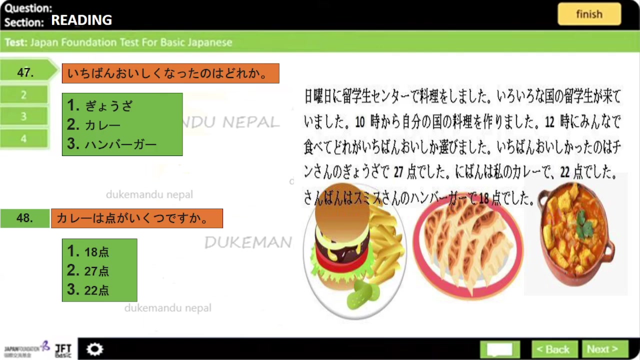 そうですか。 私は友達と映画を見に行きます。 私は友達と映画を見に行きます。 私は友達と映画を見に行きます。. 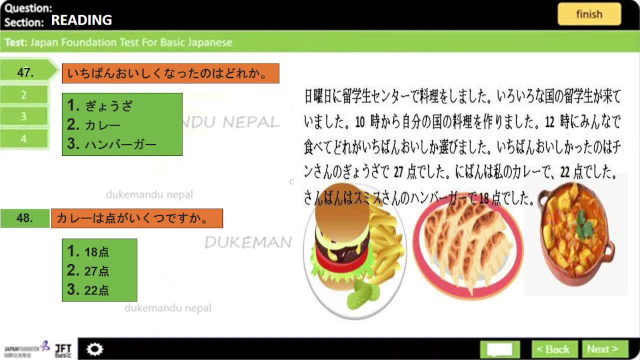 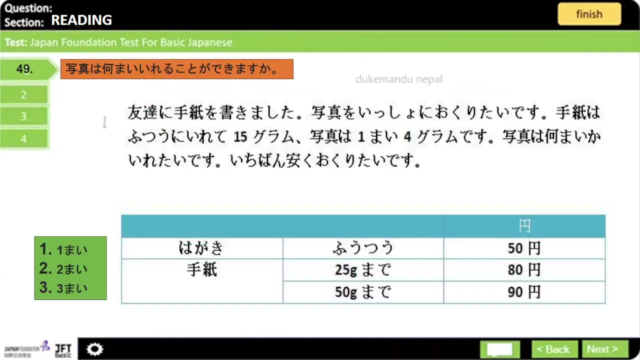 私は友達と映画を見に行きます。 私は友達と映画を見に行きます。 私は友達と映画を見に行きます。. 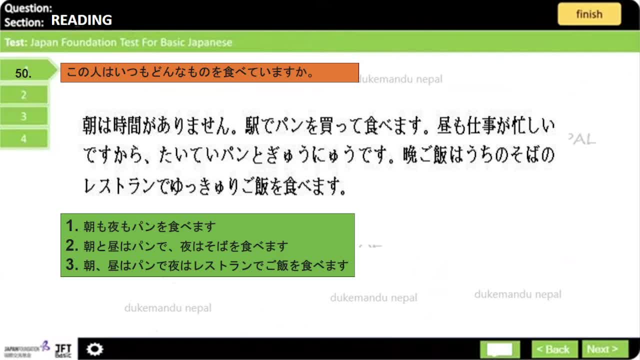 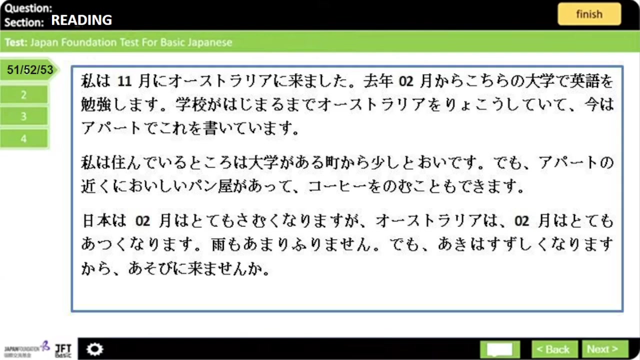 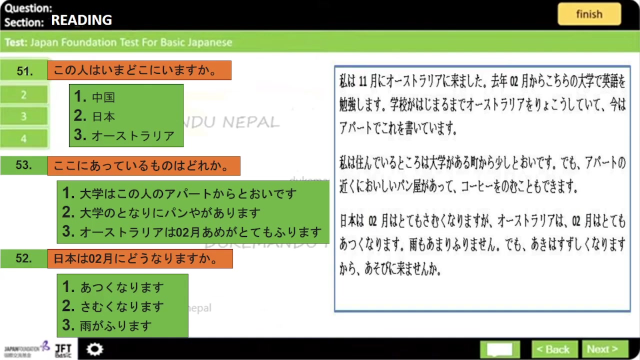 私は友達と映画を見に行きます。 私は友達と映画を見に行きます。 私は友達と映画を見に行きます。. 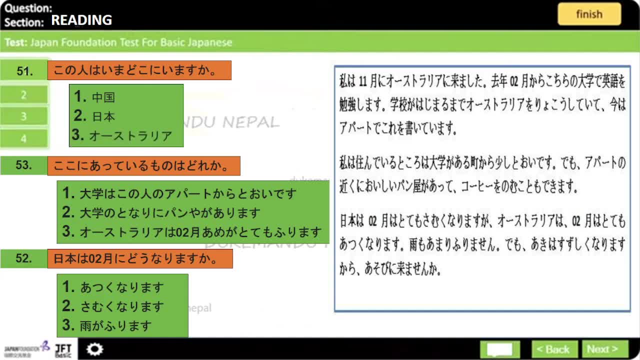 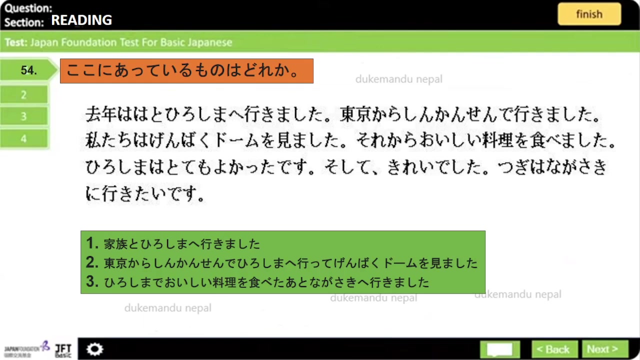 私は友達と映画を見に行きます。 私は友達と映画を見に行きます。 私は友達と映画を見に行きます。. 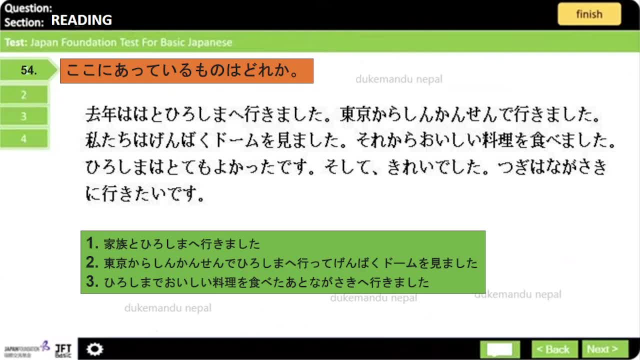 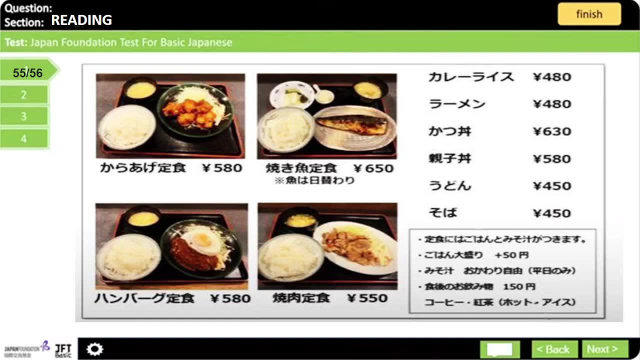 私は友達と映画を見に行きます。 私は友達と映画を見に行きます。 私は友達と映画を見に行きます。. 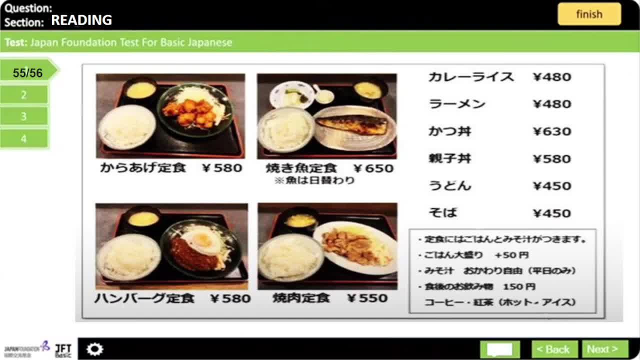 私は友達と映画を見に行きます。 私は友達と映画を見に行きます。 私は友達と映画を見に行きます。. 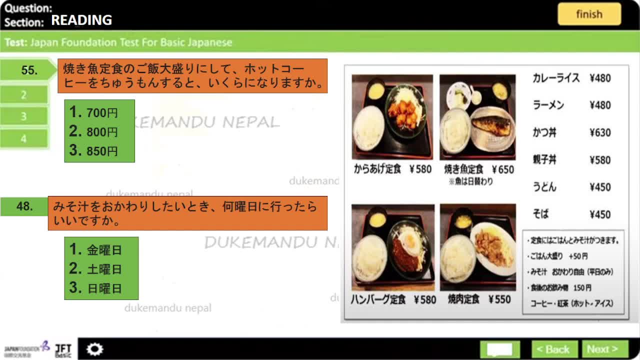 私は友達と映画を見に行きます。 私は友達と映画を見に行きます。 私は友達と映画を見に行きます。. 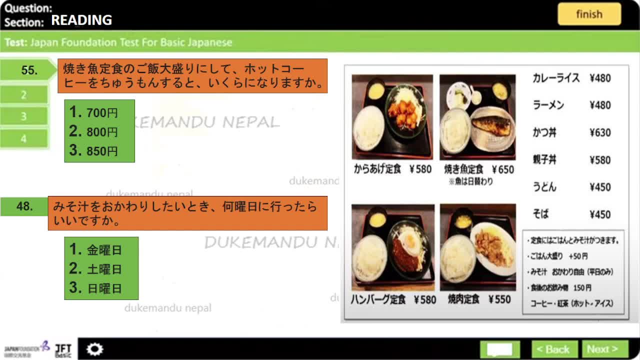 私は友達と映画を見に行きます。 私は友達と映画を見に行きます。 私は友達と映画を見に行きます。.